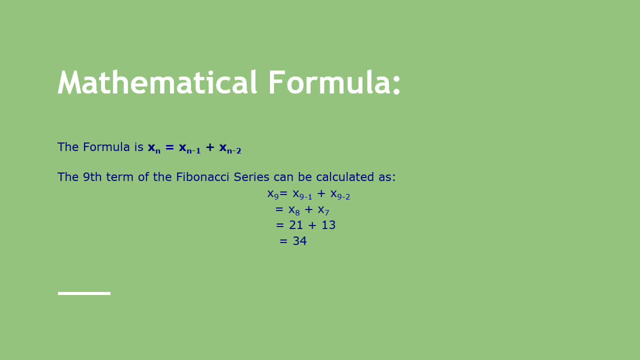 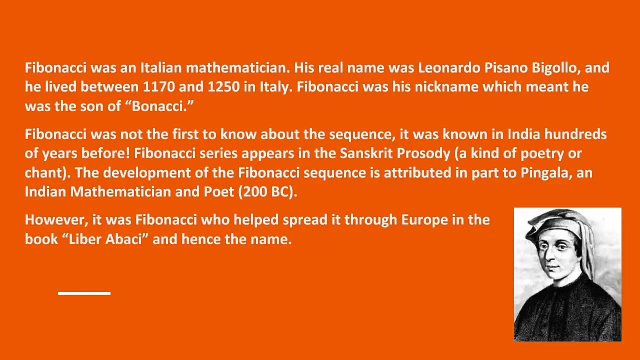 x8 is 21 and x7 is 13.. So when you add 21 plus 13,, you get x8 plus x7.. So you get x9, which is 34.. The Fibonacci sequence is named after the Italian mathematician Leonardo of Pisa, known as Fibonacci. 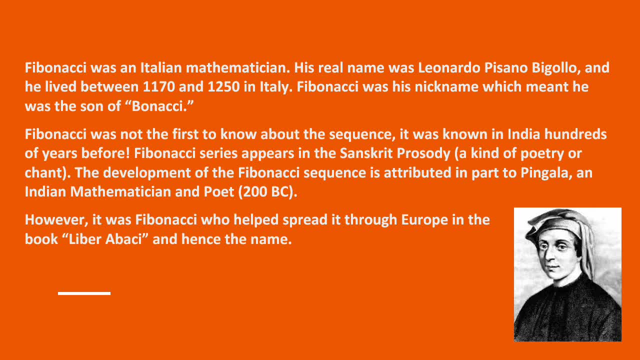 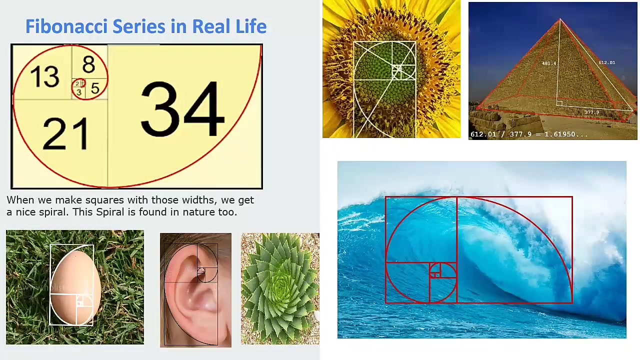 His 1202 book, Liber Abaci, introduced the sequence to Western European mathematics, although the sequence has been described earlier. in Indian mathematics The sequence appears in Sanskrit Prasodi as early as 200.. When we make squares with the widths in the series, we get a beautiful spiral. 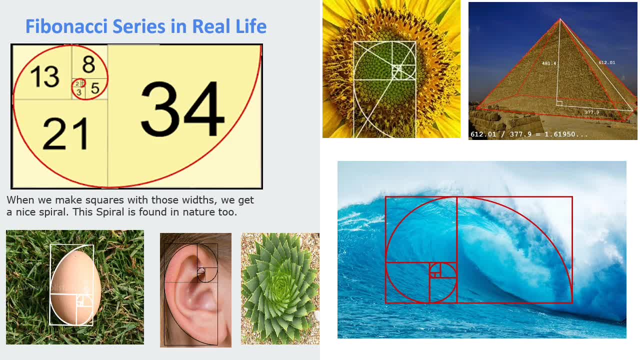 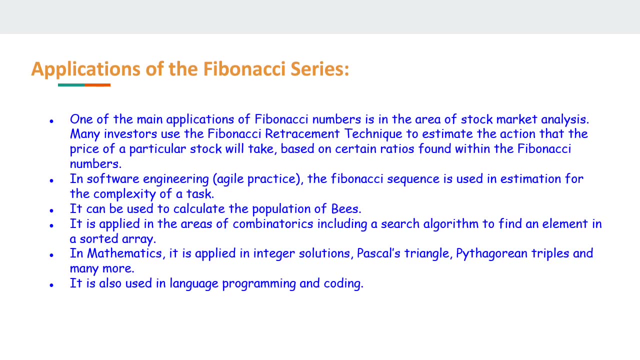 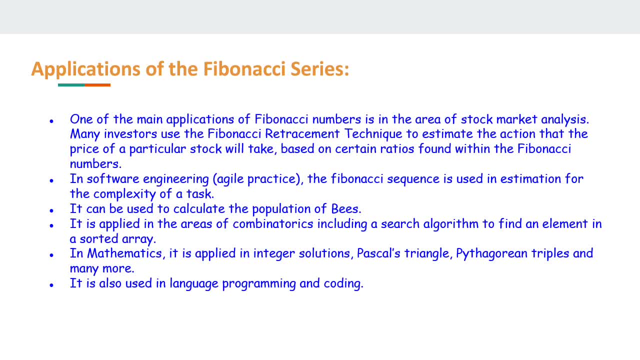 Let's see the applications of this spiral. What's a spiral? It is a part of theее. one of its main application is in the field of stock market analysis: the rise and fall of stocks. The technique used here is called the Fibonacci Retracement Technique. 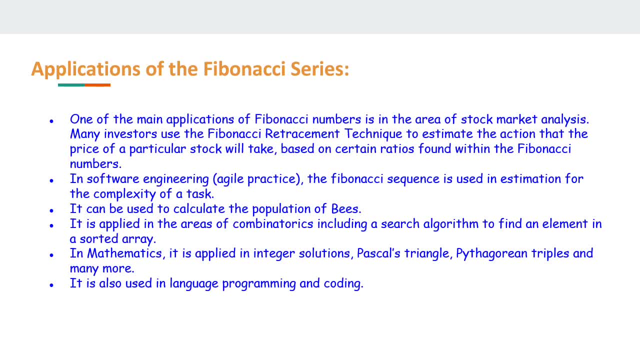 In software engineering, it is used to analyse the complexity of a task. It is also used to calculate the population of bees. It can be used in areas of combinatorics. It can be used in areas of combinatorics. In mathematics, it is applied in integer solutions. 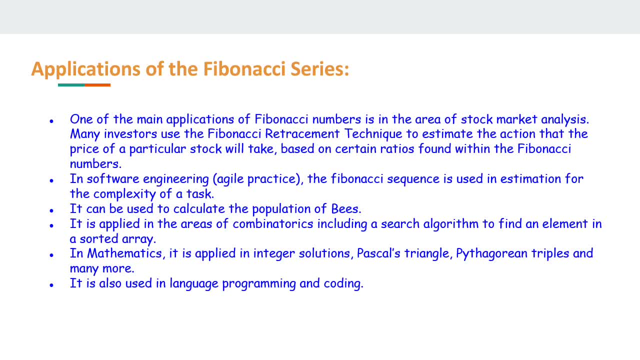 Section In马 horizon AND in English, in стом дор Paper. The first way is a sequence columns St령s. The next exercise is schem, Bolieennik equations, Pascal's triangle, Pythagorean triples and many more. 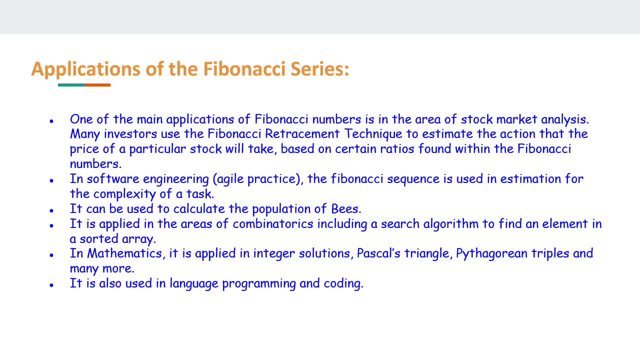 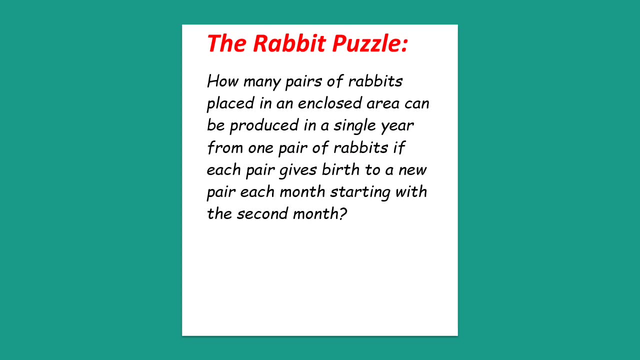 It is also used in programming and coding languages like C, C++, Java and many more. Okay, now I've got a puzzle for you. Let's see if we can figure it out. You can pause the video and try to figure out the answer.